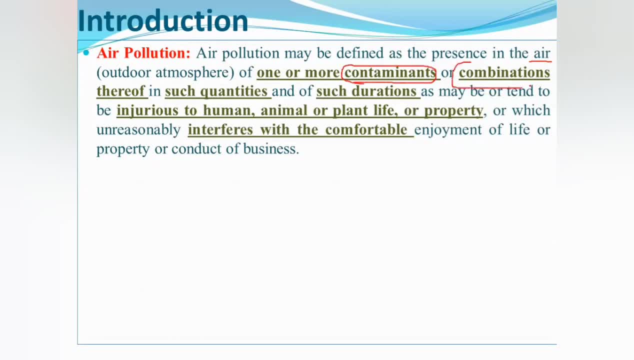 And platin. an air pollution is suppose to result in pollution or pollution in air continuity of air pollution. So what is air pollution? air pollution, The quantity should be considerable to cause air pollution. So, first of all, what is the criteria for air pollution? 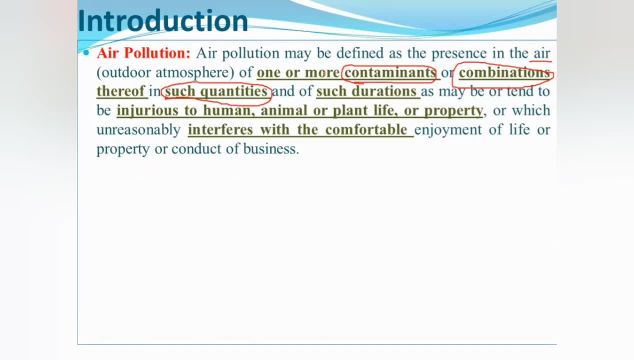 Presence of contaminants in the atmosphere and presence of contaminants in the air. Is there one or more contaminants present in the air, Or is it present in combination? And the second criteria is that their quantity should be considerable in such quantity and of such duration. 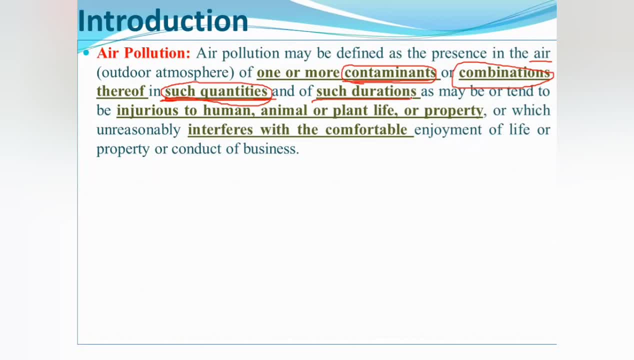 And that which is going to be present in the environment or atmosphere should be present in the atmosphere for a considerable duration. Only then air pollution can happen. This is the criteria And may be or tend to injurious to human, And its effect can be on the human being or on the animal or on the plant life, or on the property or on the buildings. 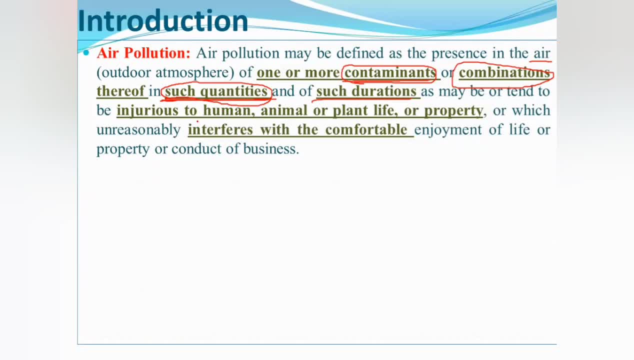 Like the impact of air pollution on Taj Mahal. Taj Mahal. So it can happen on human beings on animals on plants. So it can happen on human beings on animals on plants. So it can happen on human beings on animals on plants. 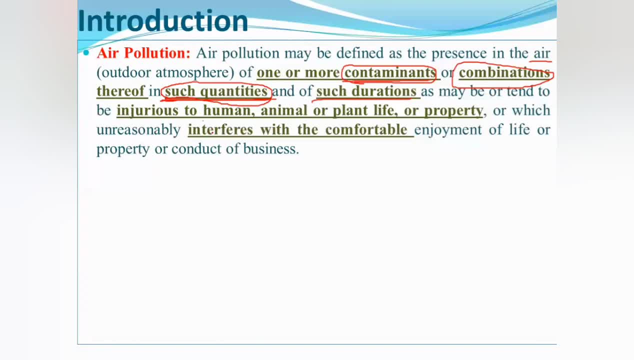 And it can also affect the property And unreasonably interferes with the comfort. Or if our comfort zone is harming the comfort, like if the temperature is very high or if the humidity is high, then our comfort zone of working cannot be achieved that much. 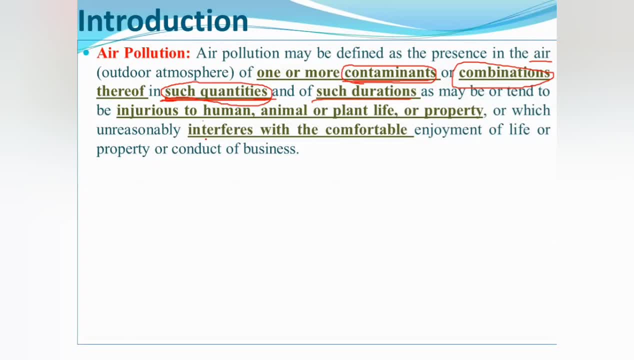 So that condition will also be unfavorable and then it will be an unreasonable condition Which will cause the enjoyment of life Okay, And property and conduct of business, Like if we have to do some work, then it can also interfere with that. 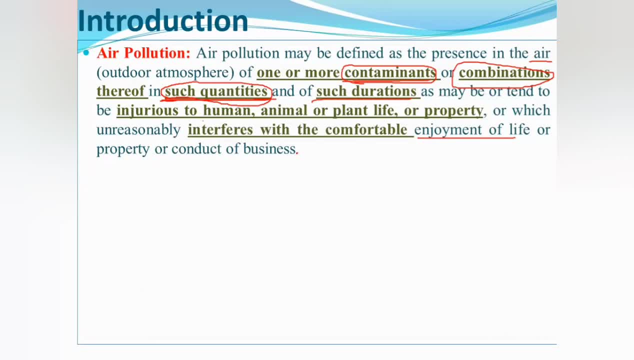 So, after all these combinations, the effect that will come, we will call it air pollution. Only one person has done combustion. Okay, After combustion, gases emit, So simply, we will not call it air pollution. When will air pollution be called? 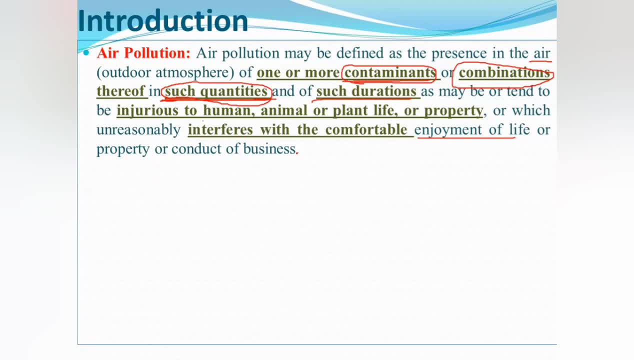 When one contaminant or more than that contaminant is present in the air in a considerable quantity, it is present for a considerable duration, And if its effect is happening on human beings, animals, plants and property, then only we will say that air pollution has happened. 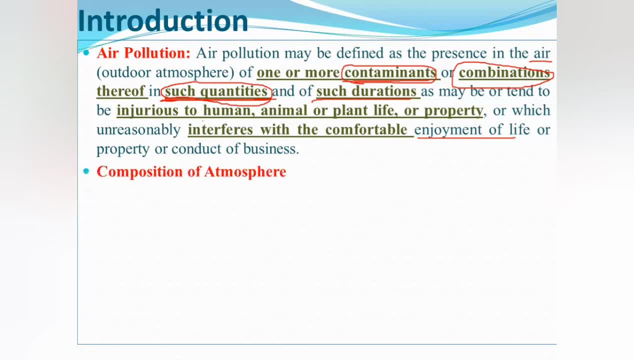 Otherwise no. I would like to give you one more example, Like composition of the atmosphere. We know that the composition of the atmosphere is 20% oxygen, 20.95% nitrogen, 78.08% argon, 0.93%. 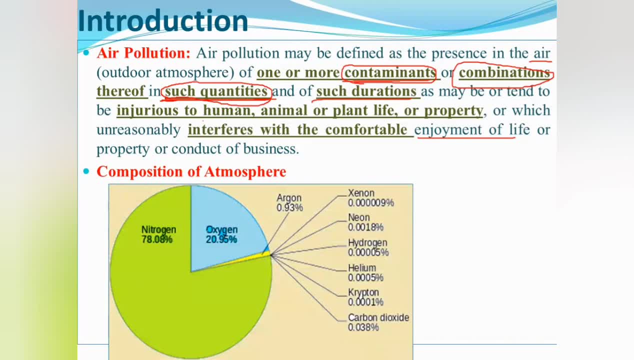 And then the other traces of gases Like xenon, neon, Hydrogen, helium, krypton, carbon dioxide and other gases. These are present in fine concentration. Okay, If the composition of all these, if the composition is concentration in the atmosphere, if it varies, if it is less or more, then we will also call it air pollution. 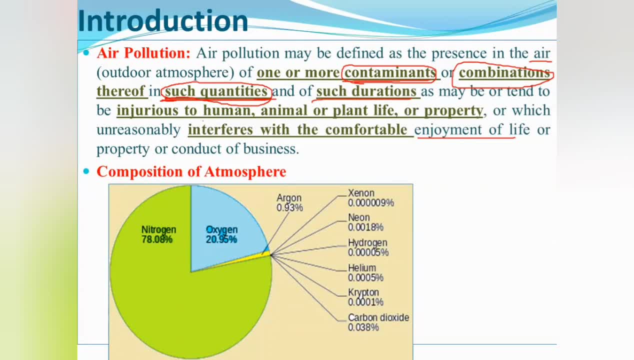 Like. if the concentration of oxygen is 22,, then we will also call it air pollution. The more oxygen is present in the atmosphere, the more it is needed. It will not work much As we say that oxygen is useful for us, But it will remain in the same percentage of oxygen. 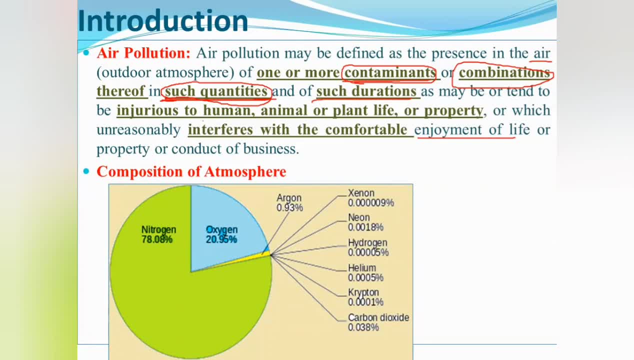 Only then it will be useful. If it is more than that, then it will not be useful. Nitrogen- Nitrogen is also 78.08%, Not much. If there is a little variation, then it will work, But not much variation is needed in all these compositions. 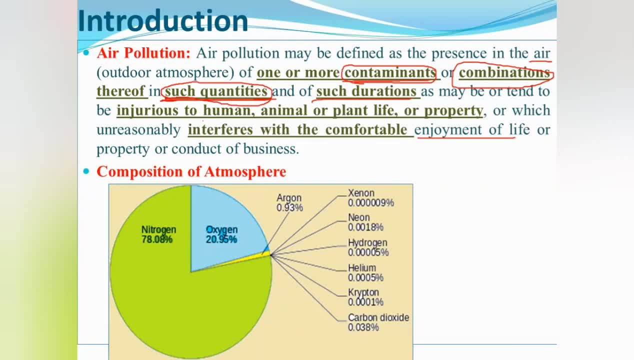 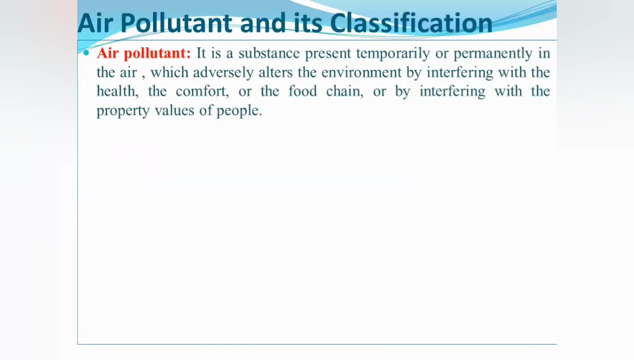 Even then, if there is a lot of variation in their composition, then we will say that air pollution has happened. Okay, I will give you more examples about air pollution. Okay, This was the basic definition and composition of the atmosphere. Then air pollutant and its classification. 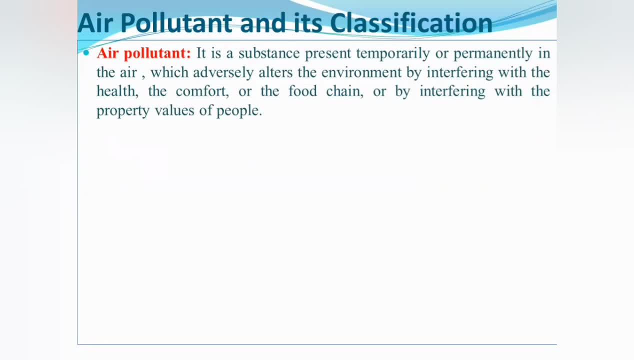 Let's see what air pollutant is. Air pollutant, It is a substance present temporarily or permanently in the air. If it is present temporarily or permanently in the air which adversely alters the environment. If it adversely affects or alters the environment by interfering with the health, the comfort or the food chain. 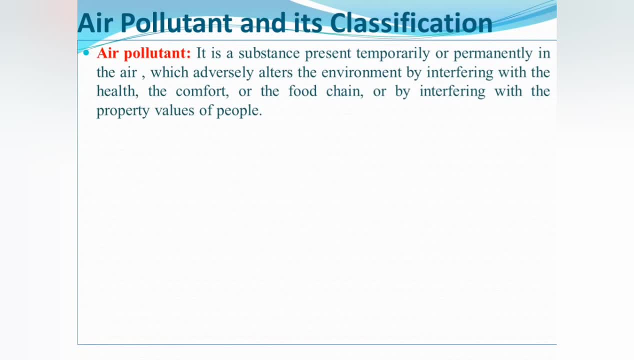 Health, The health of the human being or the comfort of the human being. Then there is food change. If there is an environmental food change, it will affect it And by interfering with the property values of the people If it affects the property, like the color of Taj Mahal is white to off-white. 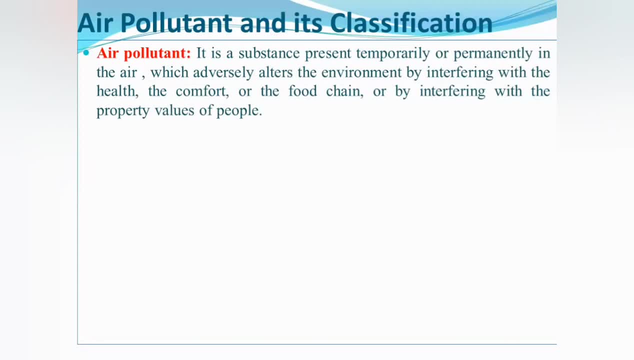 Okay, This is yellow, So that property will also be affected. Only then we will say that it is air pollutant. When the loss of Taj Mahal property is due to acid rain. What is acid rain? What is acid rain? H2SO4 is an air pollutant. 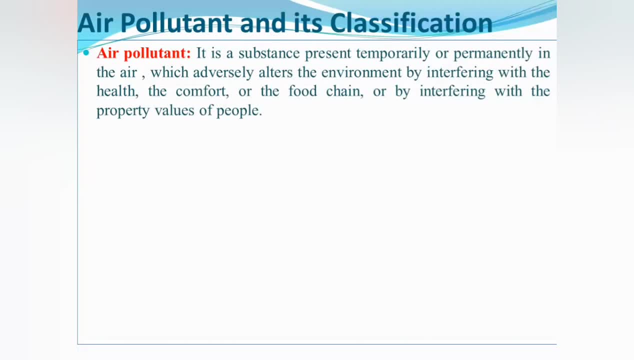 So the definition of the air pollutant is that it is present temporarily or permanently. Its effect should be in the environment, So we will call it air pollutant then. generally two classification have been done. Broadly classification will be said Primary air pollutant or secondary air pollutant. 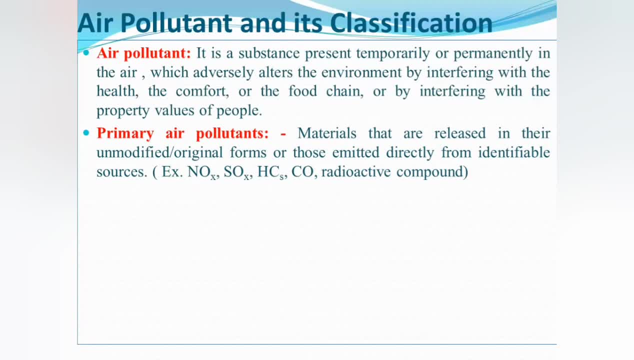 So first let's see what is primary air pollutant. Primary air pollutant means materials that are released into the air in their unmodified and original form and those emitted directly from unidentifiable sources. Primary air pollutants are such materials which are going to be directly released from the source. 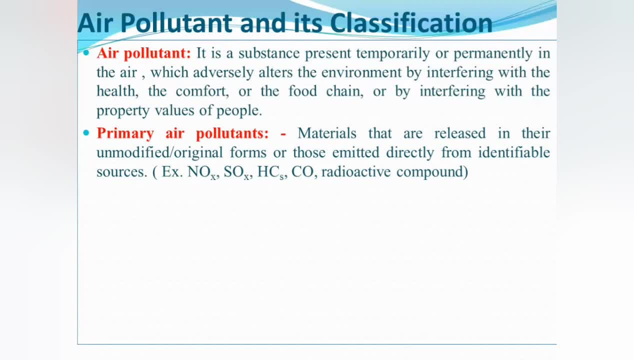 For example, combustion has carbon dioxide, carbon monoxide, nitrogen oxide, SOX and hydrocarbons which will be directly released. So these are called primary pollutants, Those which are directly released and which will remain in their original form, unmodified or original form. 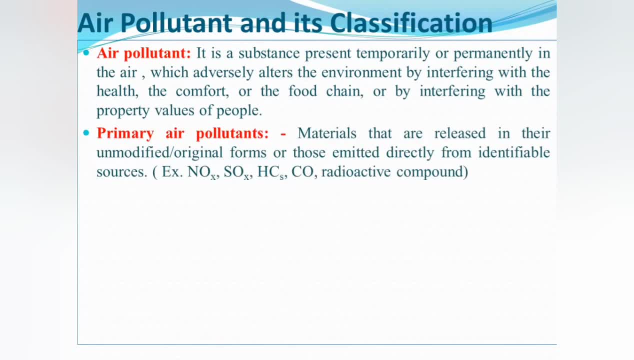 we will call them primary air pollutants. For example, NOX means oxides of nitrogen and SOX means oxides of sulfur. It means NO2, NO3, SO2, SO3 will also come- And HC means hydrocarbons. 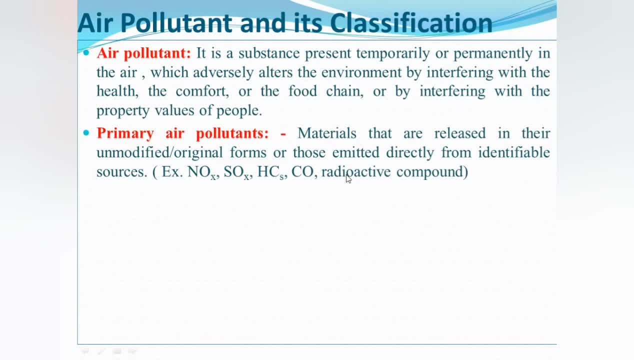 Then CO, carbon monoxide. radioactive compounds are also an example. Radioactive compounds, radioactive materials, are present in rocks. They are beneath the surface When they are decomposed. when the radioactive element of the rock is decayed, then the parent gases of the rock are released. 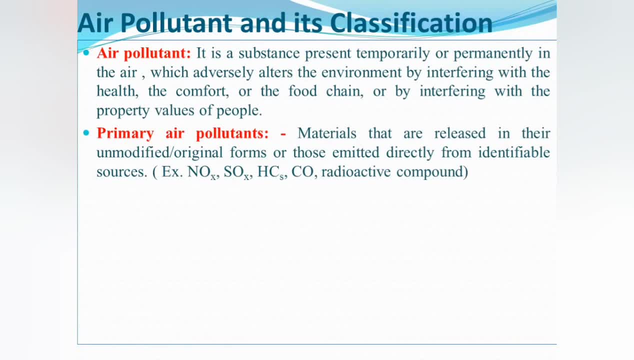 Its best example is radon gas. Radon gas comes out of the earth and is present in the atmosphere. Radon gas is an indoor air pollutant and an outdoor air pollutant, So radioactive compounds- air pollutants- can also be produced through radon gas. 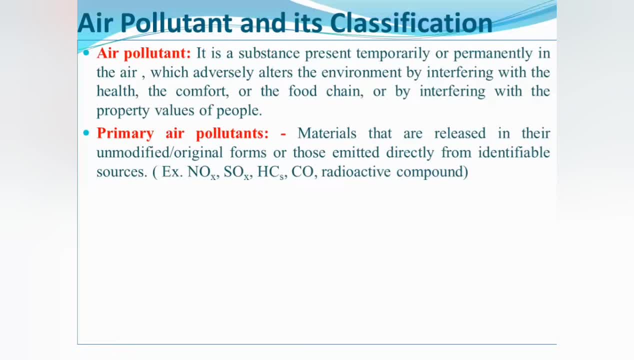 And the radioactive elements of the air pollutants that are going to come out of the radioactive compounds will remain primary Because they are directly emitted from their products. Then, secondary air pollutants. I told you about the primary of secondary air pollutants. I told you about the primary of secondary air pollutants. 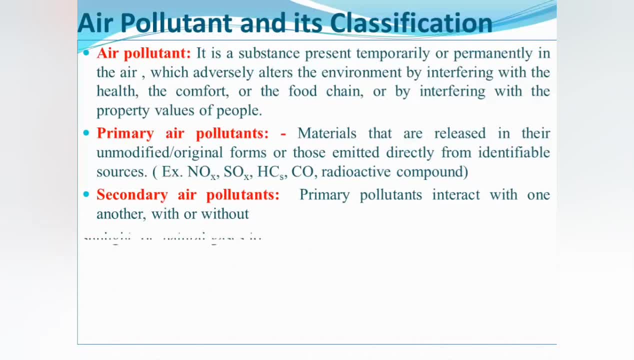 Primary pollutants interact with one another, with or without sunlight or natural gases, to produce new harmful compounds. Okay, Now what is a secondary air pollutant When primary pollutants react with one another? when primary pollutants react in the presence of sunlight or in the absence of sunlight? 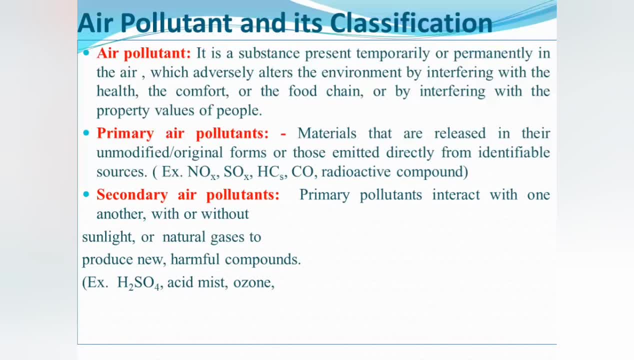 Okay, No one will say that there will be sunlight and there will be no sunlight. Okay. And natural gases? or it is reacting with natural gases to produce new harmful compounds. If a harmful compound is present, then the new harmful compound is going to be a secondary air pollutant. 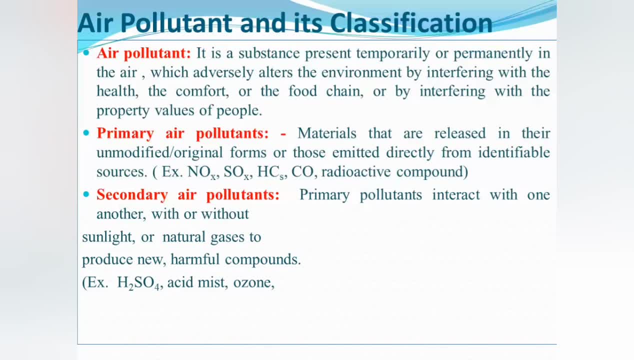 Secondary air pollutant. Its example is H2SO4.. H2SO4 is a sulfuric acid. Now I will tell you how it is formed, Or it will also be called acid mist. Okay, So when there is a combustion, 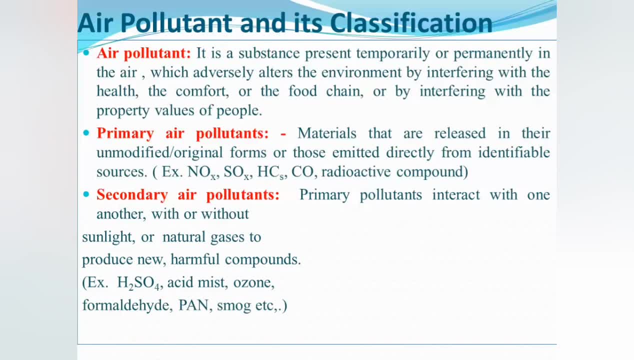 sulfur dioxide or sulfur oxides are present in the atmosphere. Okay, They are present in the atmosphere. They are dispersed in the atmosphere, Then when there is a rainfall, when there is a rainfall, then the reaction of water droplets and sulfur. 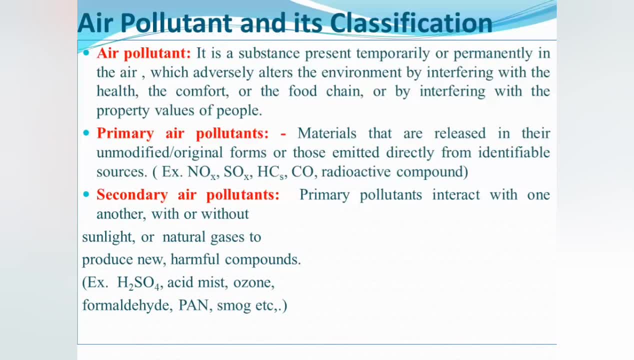 what happens to the oxides of sulfur? what happens to their reaction after they react? after they react, hydrogen- sorry, sulfuric acid. sulfuric acid is formed In this way. what happens? Acid formation. When will this happen? 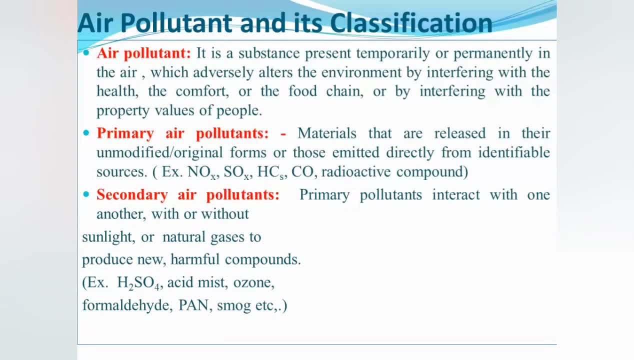 When will the acid rain form? When will the acid mist form? Okay, When will this happen? When in the atmosphere there are more oxides of sulfur, more oxides of nitrogen. If there are more oxides of nitrogen, then HNO3,. 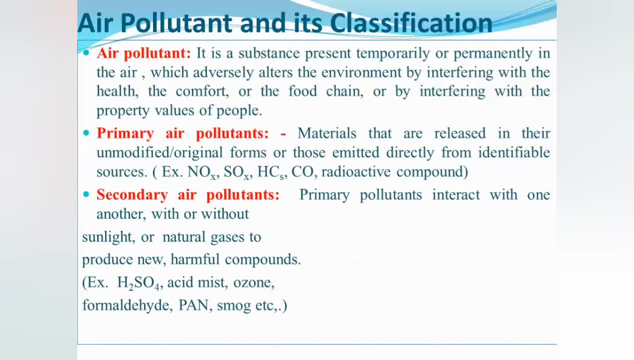 nitric acid will form. If there are more oxides of sulfur, then hydro sulfuric acid will form. Okay, So this is acid rain. When will the acid mist form? When in the atmosphere, if there is moisture in the atmosphere? 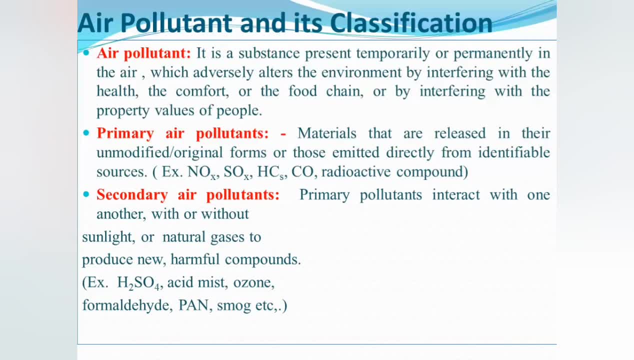 and sulfur dioxide is present, then the reaction of moisture and sulfur dioxide, the reaction of oxides of sulfur, acid will form. And what will come from that Acid? mist will come. Okay, Then ozone. What is ozone? It is a secondary air pollutant. 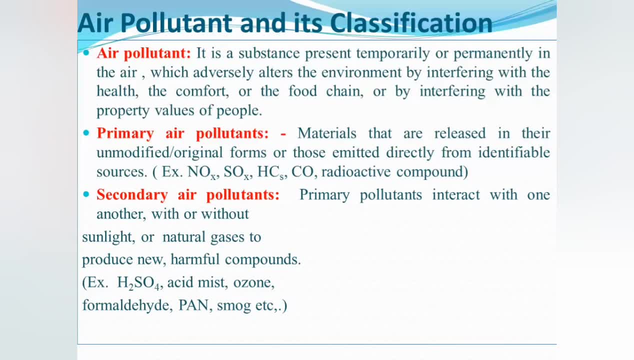 Pay attention. What is ozone? It is a secondary air pollutant. We always say that when ozone is very useful, it is very useful. But when is ozone useful? We should keep this in mind. Ozone is useful only when it is present in the ozone layer. 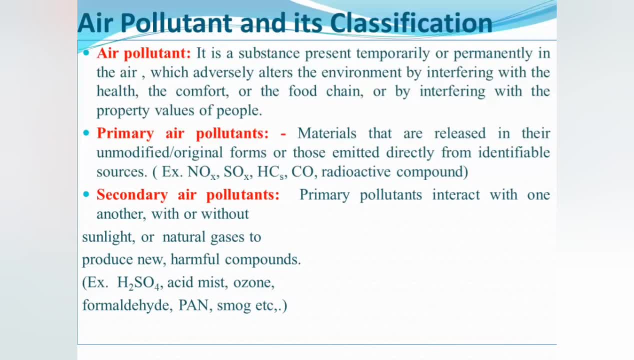 Okay, When is ozone useful? When it is present in the ozone layer. If it is not present in the ozone layer, then it is present in the troposphere. Troposphere means the layer near the earth, the layer of the atmosphere. 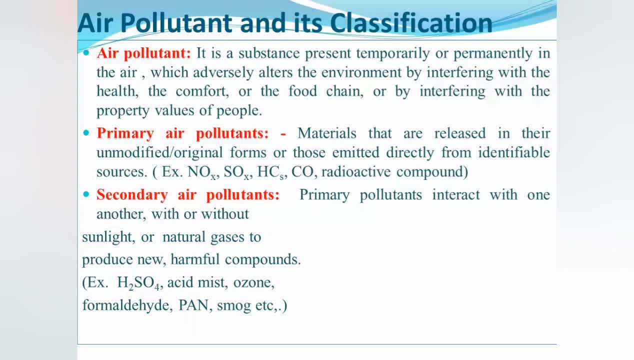 that is called troposphere. If it is present in the troposphere, then it is harmful gas. It is also a gas of ozone. Sorry, It also comes in greenhouse gas. Okay, So when ozone is pollutant, when it is present in the troposphere. 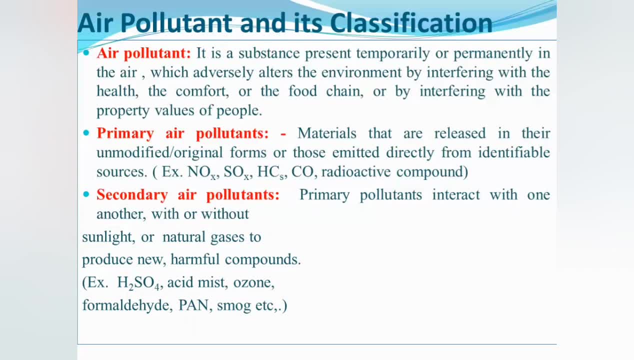 if it is present in the ozone layer, then it is useful for us. Okay, And ozone is formed by oxygen. That is why it is a secondary pollutant. Then formaldehyde, Then then, then, then, then then. 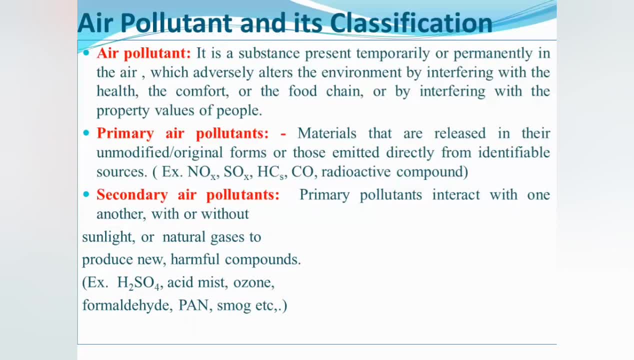 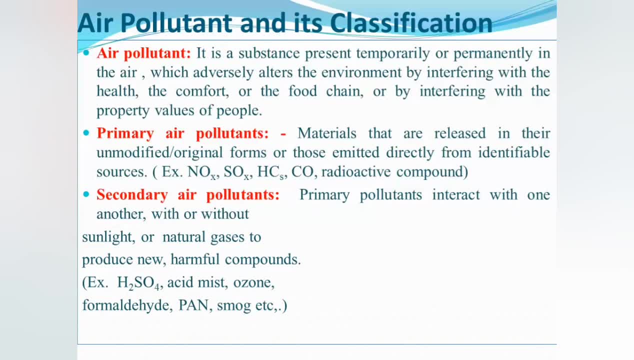 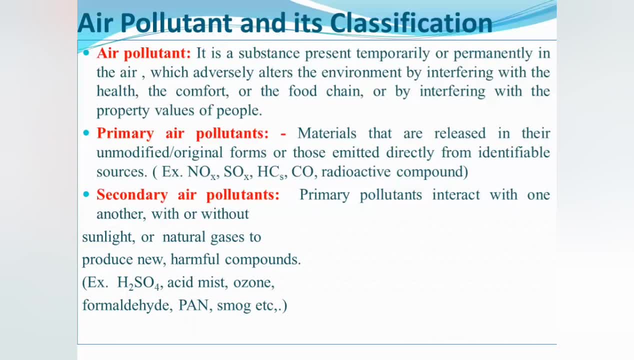 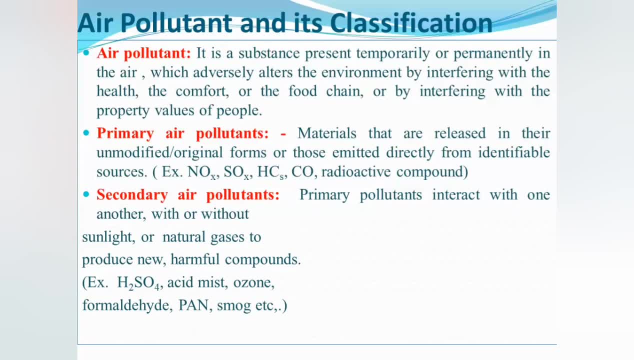 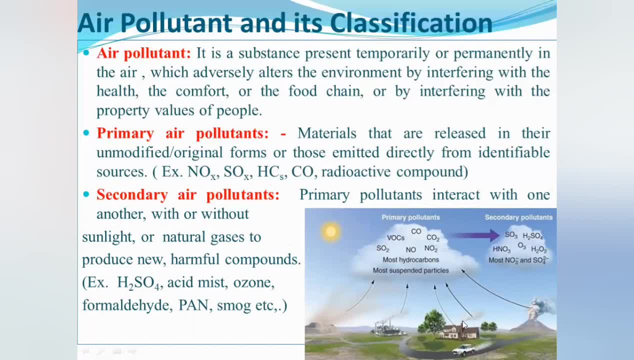 most suspended particles: Household activities which are going to be released, combustion which are going to be released. vehicle exhaust which is going to be released. volcanic eruptions which are going to be released. factories which are going to be released. desert area where dust will be very much. from there, the particulate matter, or fine dust particles. 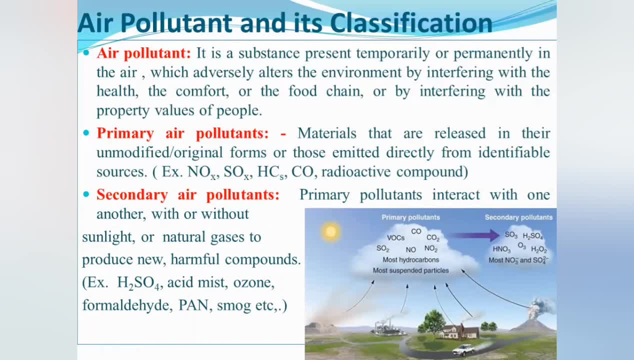 which are going to be released. all these are directly emitted by the source. So all this is primary air pollutant. Now secondary air pollutant when there is a sun rays incident on them, or in the presence of sunlight, or in the absence of sunlight, when their conversion happens. in all these, 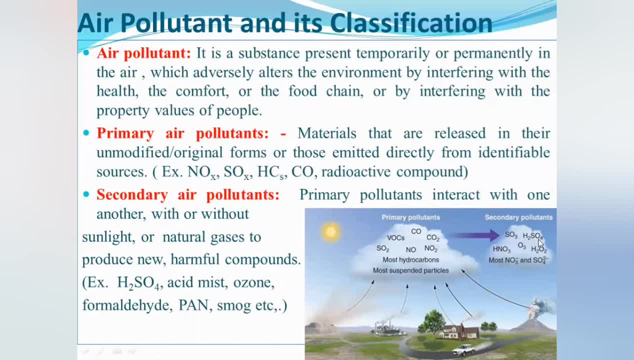 particles like sulphur trioxide, hydrogen sulphide- sorry, hydrogen sulphide, no hydrogen sulphate- Or, in the absence of sunlight, when their conversion happens in all these particles, sulphuric acid, H2SO4, HNO3, nitric acid, O3, ozone, H2O2, hydrogen peroxide- most NO3 negative. 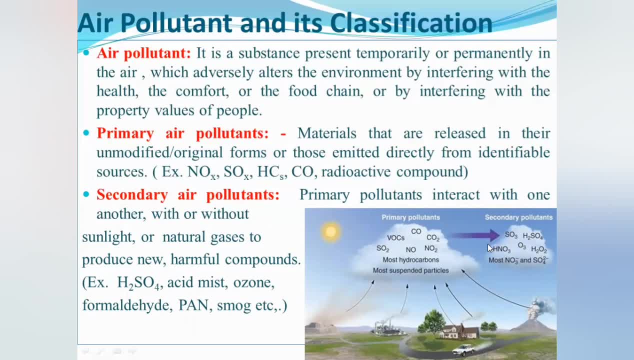 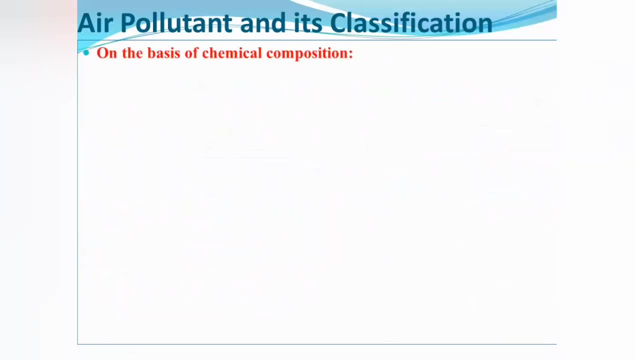 and SO4 dinegative. What are all these Secondary pollutant? What are all these secondary pollutants? They have evolved from primary pollutants. That's why they are called secondary pollutants. Okay Then, on the basis of chemical composition, there is another classification, basis of: 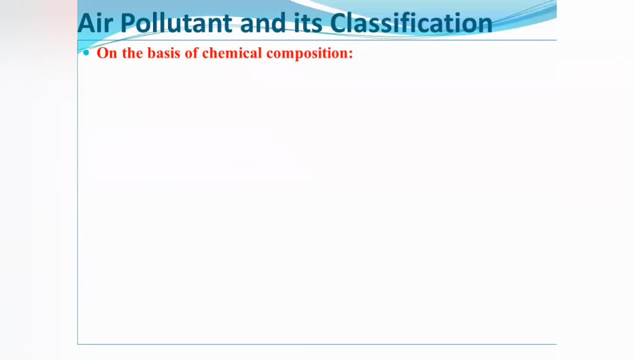 chemical composition. What is classified on the basis of chemical composition? What is classified on the basis of chemical composition? We will look at the pollutant Organic air pollutant- organic air. pollutant will be called if an organic compound is present. Organic compound contains carbon and hydrogen and, in addition, oxygen, nitrogen and sulphur. 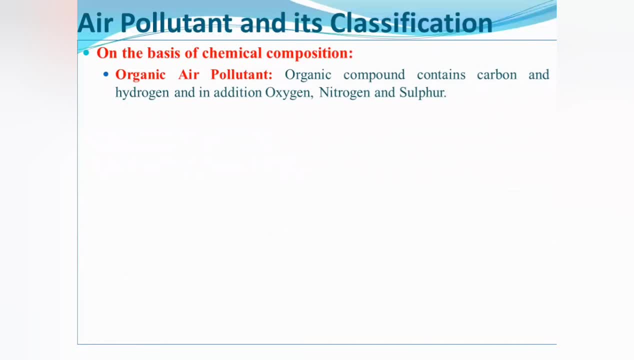 What will we call it? We will call it organic compounds. like, organic compound is made up of carbon hydrogen, C-H-N-O-S, carbon hydrogen, nitrogen oxygen, sulphur. okay, So from all these organic compound is formed. okay. 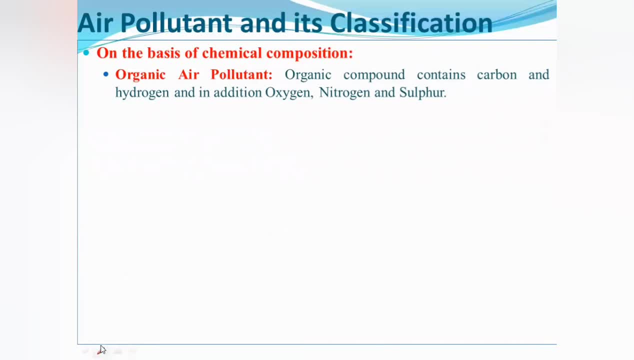 So organic compound is made up of carbon, hydrogen, oxygen, sulphur. So the major components are available in the organic compound. the major component are two: One is carbon and one is hydrogen, And in addition to carbon and hydrogen there are oxygen, nitrogen and sulphur. okay, 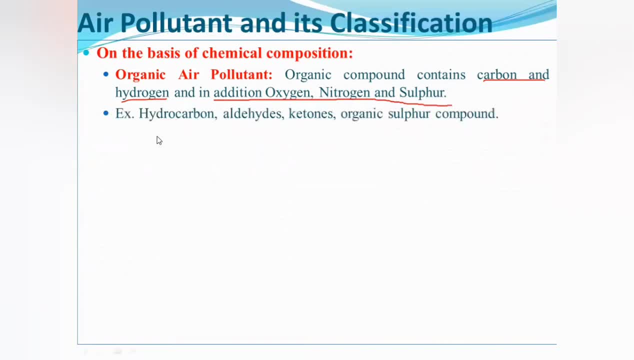 So all these are organic air pollutants. So, for example, organic air pollutants are hydrocarbon, aldehyde, ketones, organic sulphur compounds. What are all these Organic components and organic air pollutants? Ok, Okay, Ok. inorganic air pollutant- inorganic air pollutant, con con say it includes: 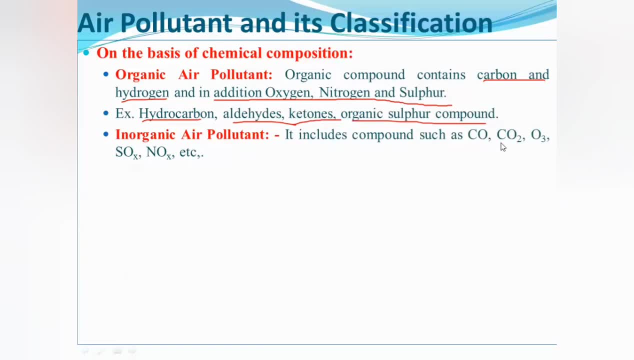 compounds such as co, carbon, carbon monoxide, co2, carbon dioxide, o3, ozone, oxides of sulfur, oxides of nitrogen, etc. okay, so, yes, a big a inorganic compound of organic compound may be a palatable, a carbon which I, a hydrogen which I or hostess at, may occur oxygen at run. sulfur had a cherry either. they can see. 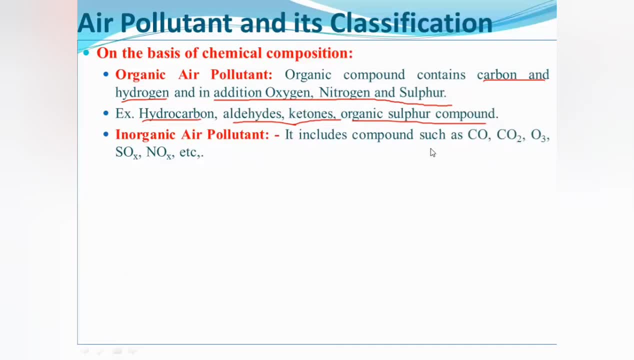 carbon oxygen. either we see carbon oxygen either be syrup oxygen and to in organic compounds at east is probably the market sector, at rock sector. then, on the bit, on the basis of state of matter, state of matter in a conscious state, my present away, solid state, my present, I guess a statement present a liquid. 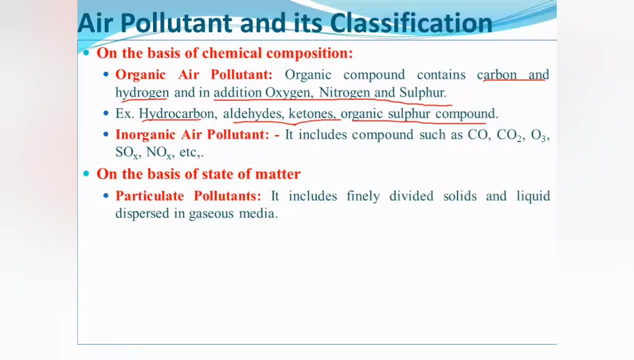 statement present a loses up to be cackey. a classification key again. the pilot classification houses of a particulate pollutant. particulate pollutant means it includes, you can see, inorganic air pollutants, inorganic air pollutants, inorganic air pollutants which finally divided solids and liquid, liquid or disval dispersed. 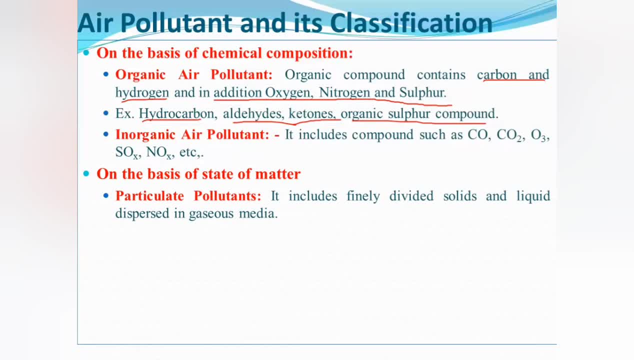 in gaseous media, gaseous mediani atmosphere, atmosphere, maybe a solid liquid finally divided. so holy dear liquid particles are present, Arvatan unterwegs around particulate pollutant, because I'm kitchen, so particulate pollutant may be. though ty� a salida particulate pollutant or Dua liquid. 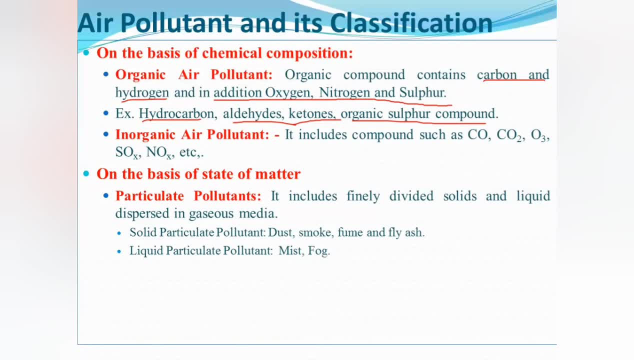 particulate pollution, solid particle pollutant J. who is coming? a simple data just In Delhi, pollution level will be very high. In that time you must have heard in the news that PM10, PM2.5, PM5 values have changed, Or PM10 value is very high, PM2.5 value is high, PM5 value is high. 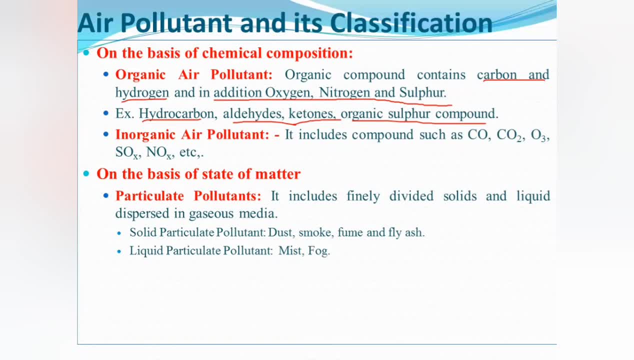 This is particulate matter. This particulate matter can be either fine, solid particulate pollutant or liquid particulate pollutant. The example of solid particulate pollutant is dust Fine. dust, fine particles of soil are dispersed in the atmosphere. If they remain suspended in the atmosphere then it will be called particulate pollutant. 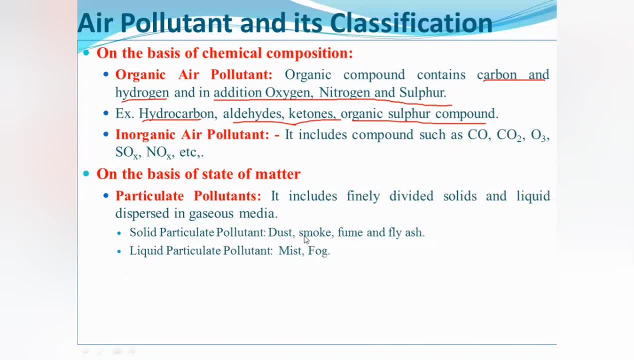 Smoke. smoke is also a type of smoke, But it is a harmful, unpleasant and unwanted fume. The smoke that is going to be harmful, we will call it fume. Generally, if combustion is done in industries or if hazardous waste is combustion, then the smoke that will come out of it, we can call it fume. 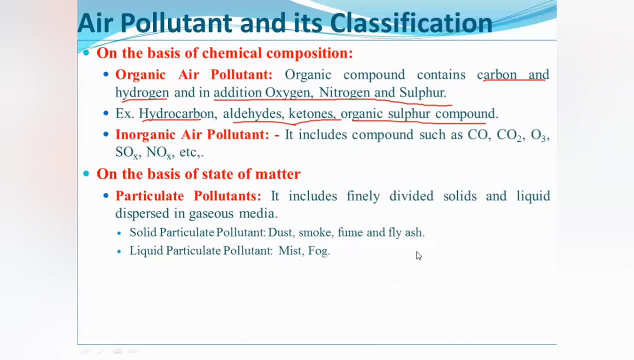 Then fly ash, like coal or any coal or thermal power plant. When combustion is done, fly ash is generated and it remains. very fine What happens in the air? It keeps getting dispersed in the air. It can go from one point to another point in the air. 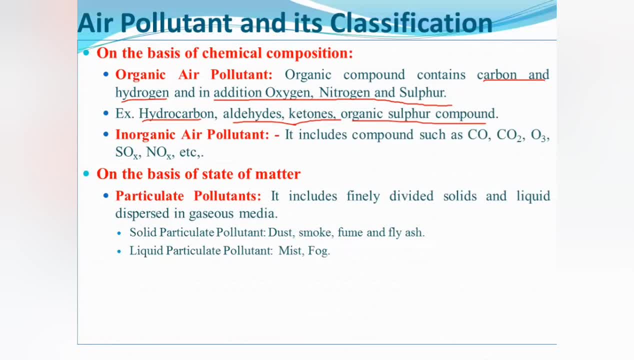 Because it remains very fine, And that is also a type of air pollutant. Now, when I told you all this, I told you solid. Then what is liquid particulate, pollutant Mist, fog, Mist and fog. Both are the same. 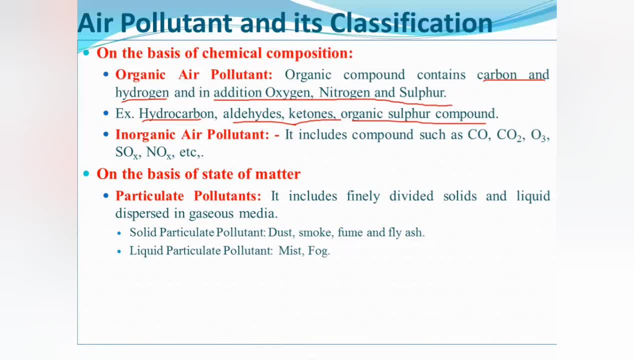 As we will say, quora. If water molecules are present in the atmosphere, then we will call it mist or fog. What is fog? The difference of these two will be seen according to visibility. If there is a quora or if the visibility is low, that is, if the fog is present or if the water molecules are present in the atmosphere. if we can see up to 1 km, if the objects are visible in it, then it is fog. 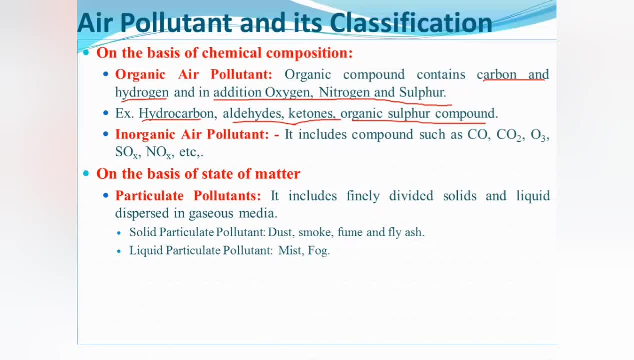 If we can see up to 1 km, then it will be called fog, Or if we can see less than that, it will be called fog. If we can see up to 1 km, then what will we call it? In the atmosphere, what is prepared? what will we call it? 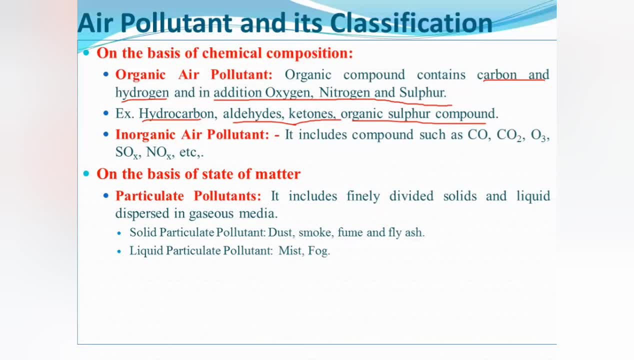 We will call it mist. What are those two? Water molecules are present, but the visibility affects visibility. So this was liquid particulate matter, Then gases pollutant. Now, what are gases pollutant? These are organic gases such as CH4.. 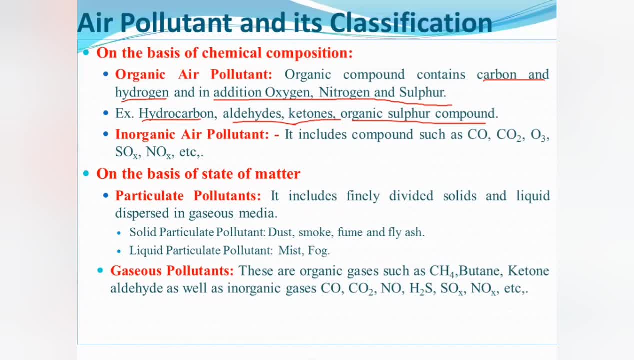 As I told you at the time, what is important in organic matter? Carbon and hydrogen, Oxygen, nitrogen, sulfur will work, but it will not work. Then butane, Cyanide, C2.. C4H10.. The formula will be whatever it is. 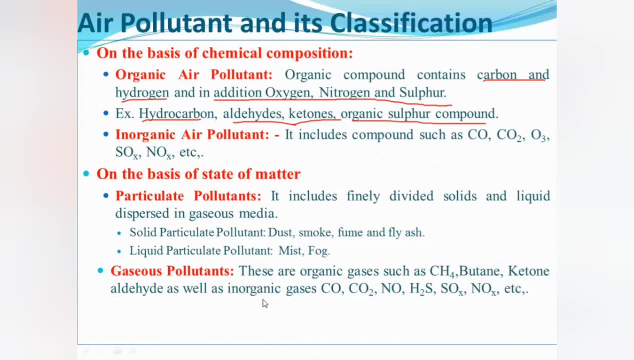 Then ketone, Then aldehyde, As well as inorganic gases. There are also inorganic gases like carbon monoxide, carbon dioxide, nitrogen oxide, hydrogen sulfide, oxides of sulfur, oxides of nitrogen and etc. What are all these? 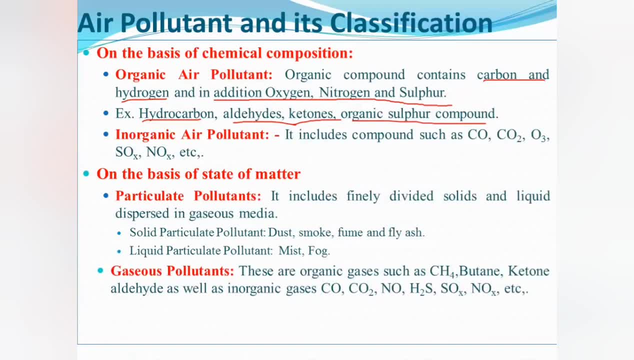 Gases pollutant. Now one example I have not mentioned here. This is particulate pollutant, And particulate pollutant is also like this: It is classified as a respirable particulate matter or a suspended particulate matter, The particulate matter that we can inhale. 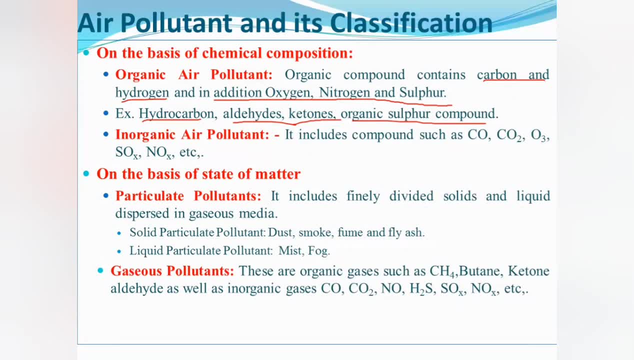 The particulate matter that can go to our lungs. We can respire. What will we call it Respirable particulate matter, And what we cannot do is suspended particulate matter. What are they in size? They are airy, Okay. 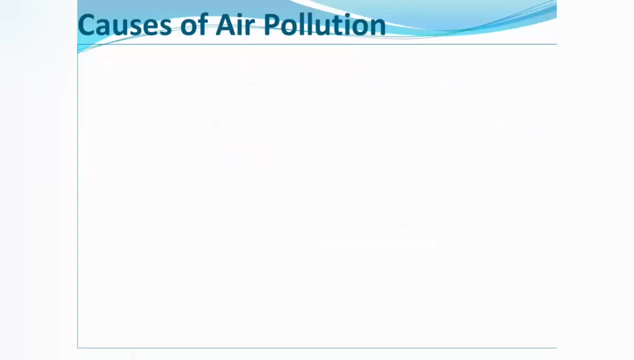 We will see its size in detail later. Then, causes of error, Causes of air pollution. What are the causes of air pollution, or sources of air pollution? First is natural air pollution. Now, what are the causes of natural air pollution? Forest fire. 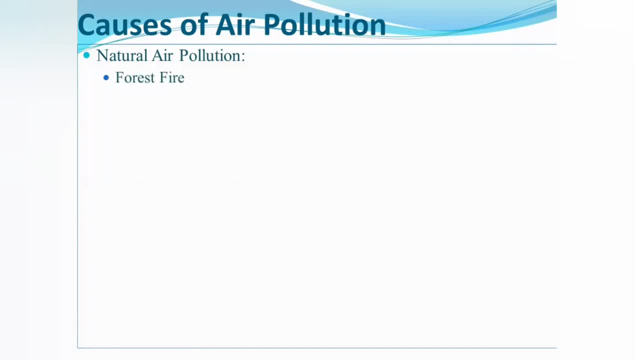 If there is a fire in the forest, then it is going to be natural. If it is a human being, then it is a different matter. Okay, If there is a combustion in the forest, then if there is a fire in the forest, then the pollutant will rise in this. 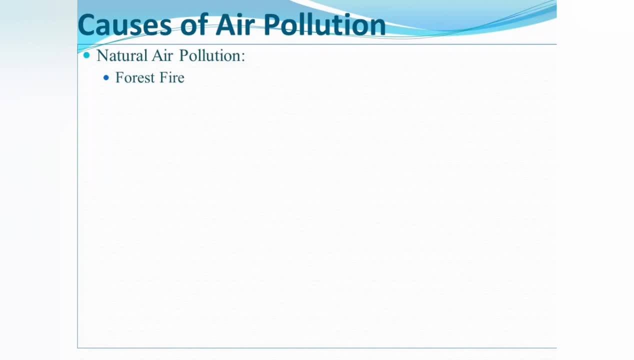 Now in the forest there is a lot of fire. In the last year there has been a lot of fire in the Amazon forest. There has been a lot of fire. What is called The greenery area has been completely combustion. 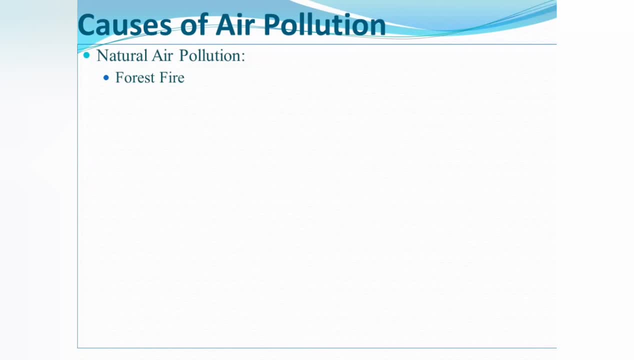 Due to that, the air pollutant is very much emitted. Due to that, the impact has been very much on the environment, Because you know such a big forest- It is a very big forest, So there are so many plants there. 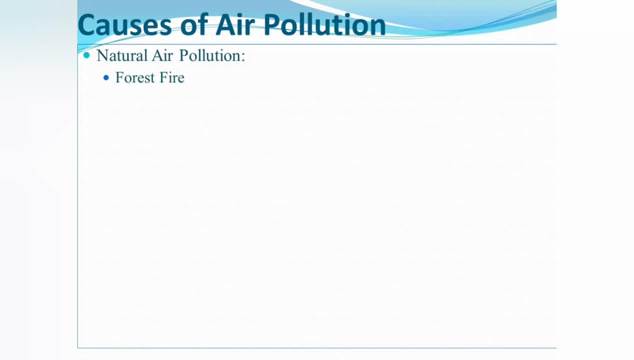 That is, they have burned and due to that, air pollutants were released in atmosphere. that was an example of natural air pollution. then volcanic eruption: volcano eruption is also a natural process. it is not through us. when volcanic eruption happens, fine, suspended particles are also released, gases are also released. 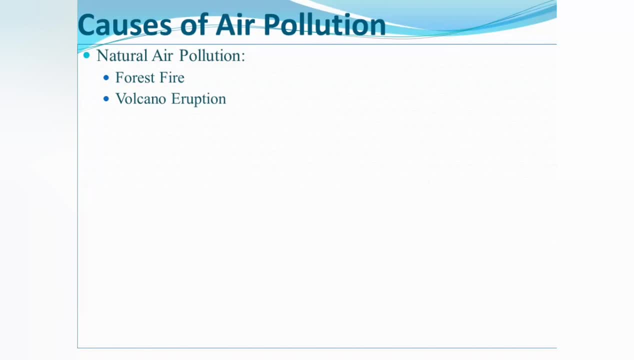 this is also an example of natural air pollution. then gases released from radioactive decay of rock. as I told you earlier, if radioactive element decay or in the form of rock gases are released and commonly known gas is radon gas, these are all examples of natural air pollution. 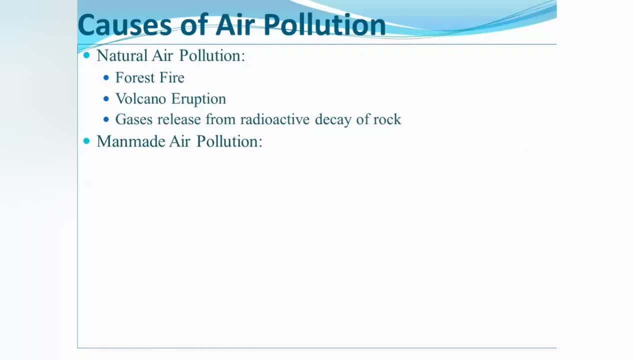 then manmade air pollution. we can do anything. we can do anything anything people do. that involves burning anything people do. that involves burning, using households or industrial chemicals, that producing large amount of dust or gases. any activity we do and due to that activity, large amount of dust. 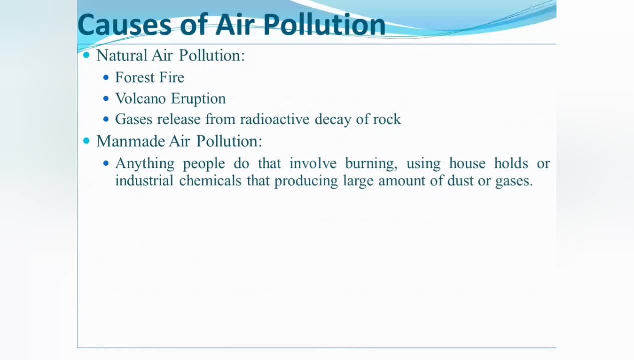 large amount of pollutants will be released in atmosphere. that will be manmade air pollution. we will see examples of that. traffic and vehicles transportation activity or traffic. so we need vehicles for transportation and vehicles are all children's vehicles. two wheeler, four wheeler use petrol. 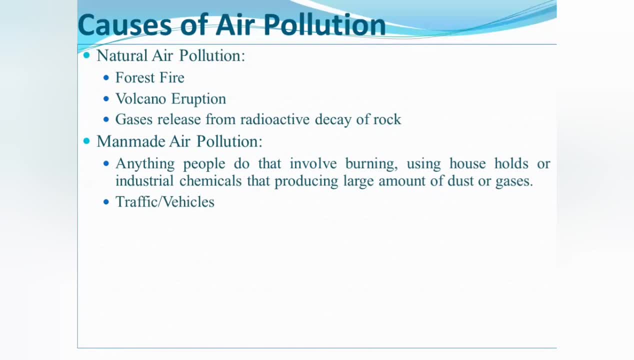 diesel, gasoline, etc. so they use fuel. fuel is made of combustion, after combustion, the silencer, or exhaust gases. the exhaust gases are released from the silencer, so in that the main components are co, NOX, volatile organic compounds, lead. So this is also a source of air pollution, but it is manmade air pollution because human beings are doing this activity. 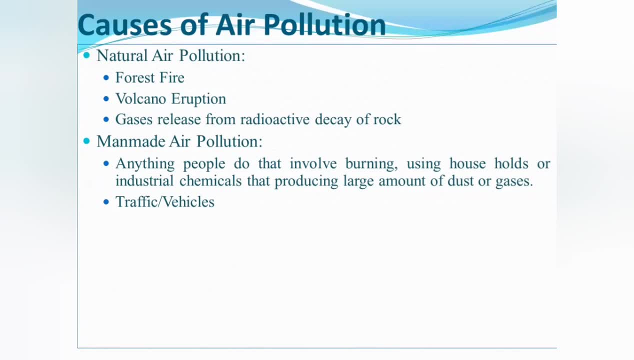 So what is done is that the PUC of our vehicle is checked. The PUC is checked to see the level of pollution due to our vehicle. While checking the PUC, if pollutants or contaminants are emitted in the atmosphere, then we do not get PUC. 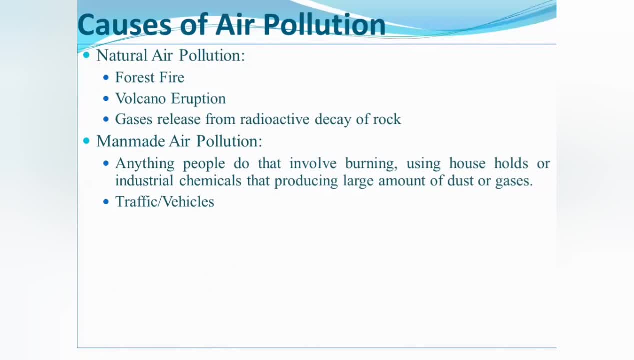 So what we have to do at that time is to change the engine or do maintenance of the vehicle. Then after that, power plants. Power plant is an example. Most power plants have power plants. Most power plants use fossil fuels. This is an example of a thermal power plant. 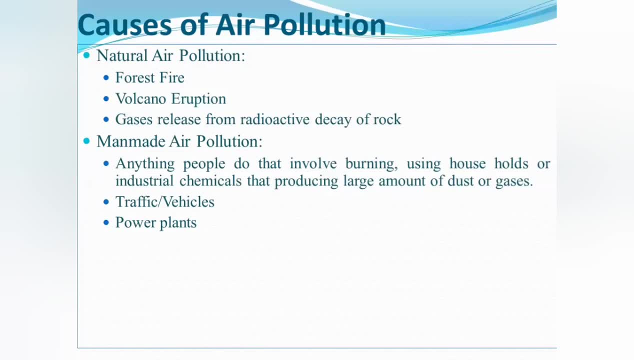 In a thermal power plant, coal is used, Sometimes steam is generated, Gas or oil is used. So when these are going to burn, What is it called? When coal is burned, the pollutants emitted from it are going to be very much polluted. 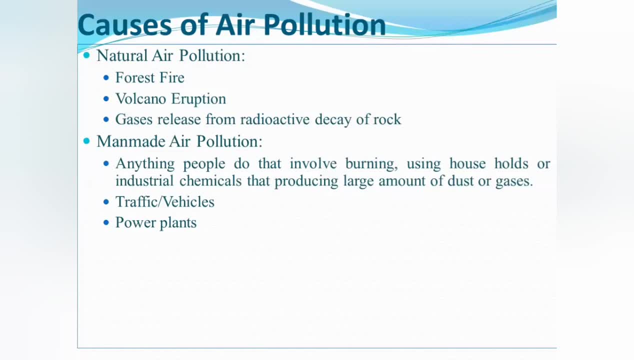 Because there are fossil fuels, Fuel is used, So pollutants are going to be emitted there. So after that, Next is industrial plants and factories. Now in industrial plants and factories like steel, aluminium refineries or petroleum producing industry, 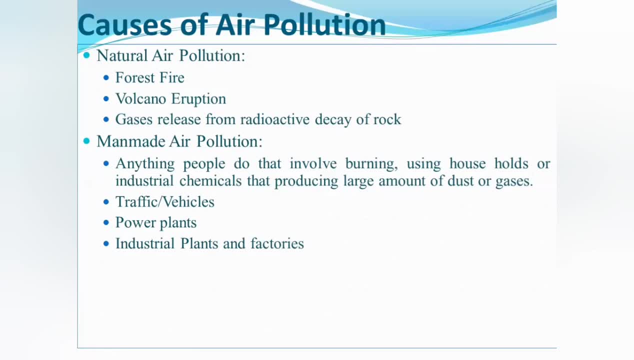 or cement industry, or stone crusher industry, Right, So all these industries have different activities. Now what will happen if different activities are going to happen? Different things are going to be produced. Pollutants can be produced, Then other causes of air pollution. 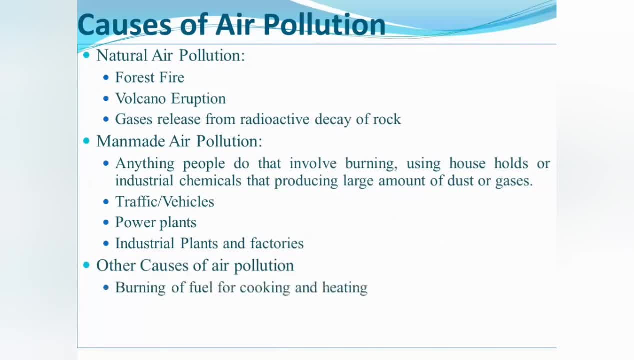 What are the other causes of air pollution? We will see that Burning of fuel for cooking and heating- We have to burn fuel. for cooking or heating, We have to burn fuel. So now this is used in very few places Like what we used to do conventionally in villages or cities. 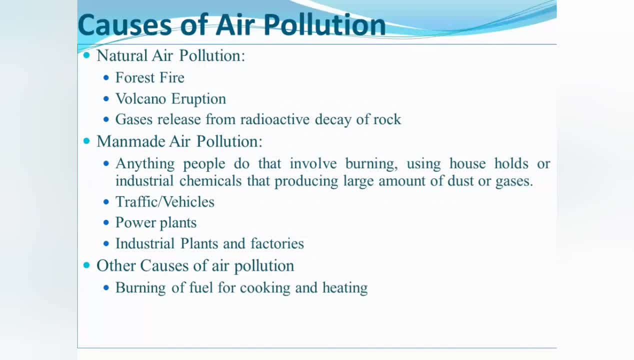 What used to happen earlier. Wood is used for cooking. Then what is used for heating? to heat water, Wood is used. What happens because of that? The air pollution is very high. It used to increase because gases used to emit more. 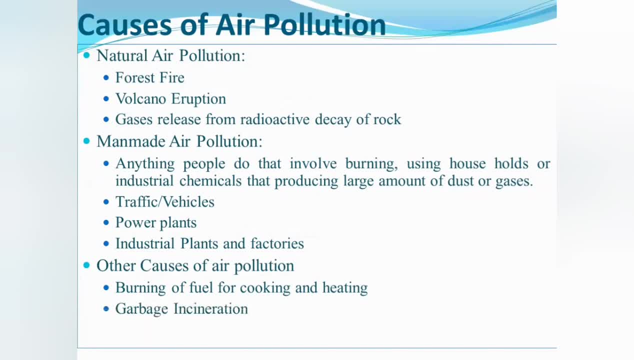 So this is also one of the causes of air pollution. Then garbage incineration: If we are not dumping garbage, solid waste, properly recycle, reduce, reuse. if we are not doing it, then if we are incinerating it directly. 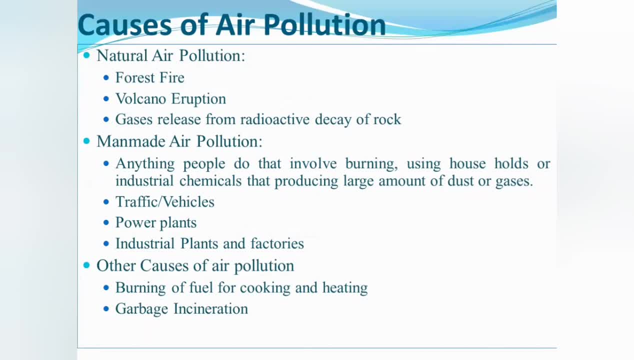 then what can happen? because of that, Pollution level can be high Because even after incineration the conversion of solid waste will be in gases. Then those gases will become pollutant after coming into the atmosphere If garbage is incinerated. 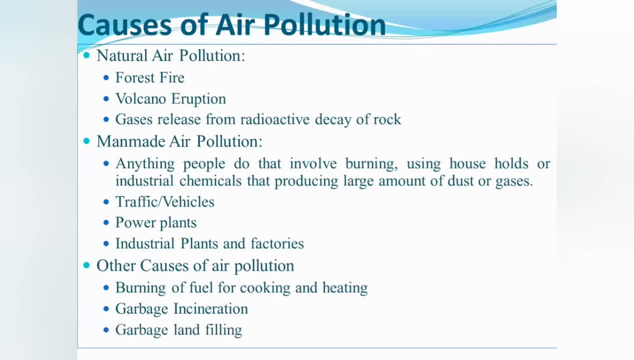 Or if garbage is filled with landfill, then how can it happen after filling with landfill? I will tell you When we are filling with landfill, then what happens after filling with landfill That it is in an aerobic condition. What is land filling? 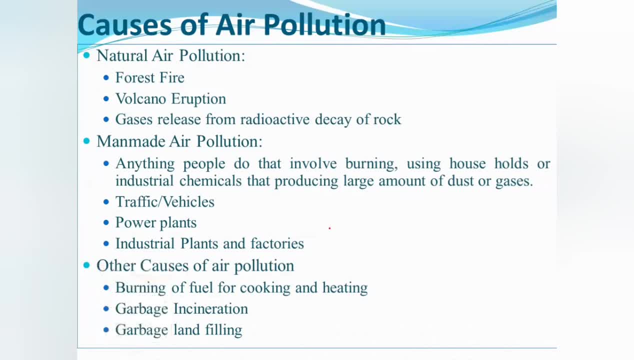 Suppose 2 minutes. Suppose there is a ground level. What is land filling? An excavation is done. What is done for this portion? Excavation is done Now, after doing so much excavation, the solid waste is dumped in this proportion. 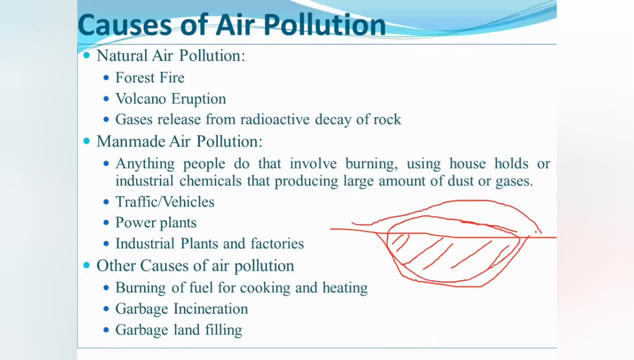 After dumping here, it is provided with cover. What is done on this? Cover is provided. Now, what happens after providing cover? What is the condition inside it? What is the condition inside it? It is an aerobic condition. Now, what will happen due to an aerobic condition? 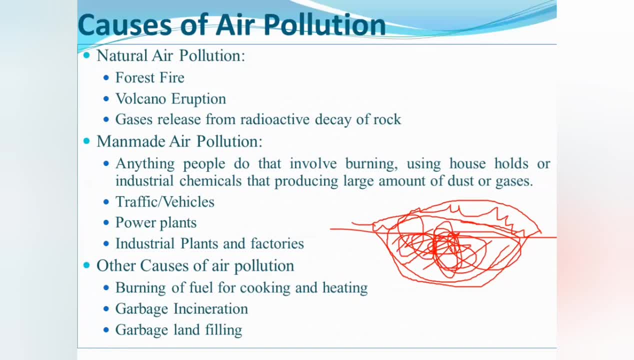 There will be an aerobic digestion. Due to an aerobic digestion, what will happen? Carbon dioxide or methane formation will be more. What will happen due to the formation of methane? What will happen? That the methane, that methane, will be present in the atmosphere. 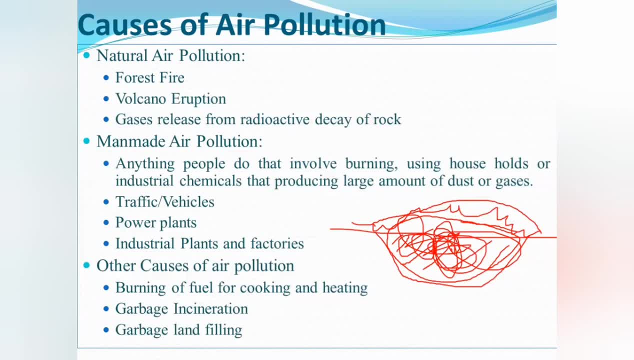 Now, if methane is present in the atmosphere, then the greenhouse gas of methane. due to this, what can happen? Air pollution can happen Even after doing land filling, because gases which are going to come up from the ground if it is not treated by collecting it properly. 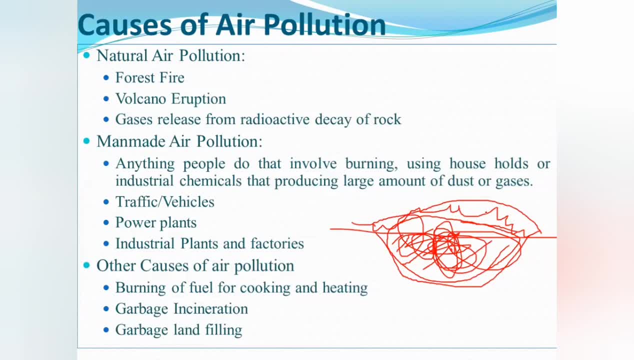 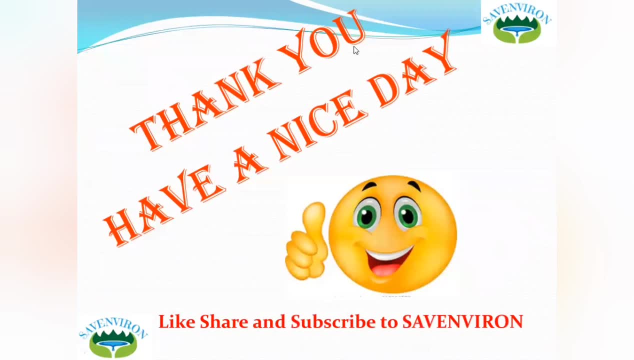 then it will come in the atmosphere. Due to this, what can happen? Air pollution can happen. So these were all the causes of air pollution. Thank you and have a nice day. Thank you.